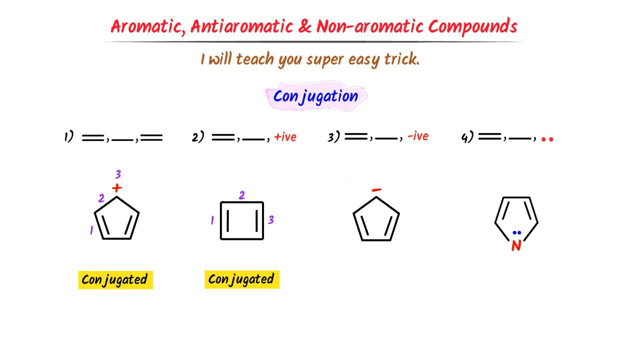 single bond and a negative charge. I write 1,, 2,, 3.. This organic compound follows the third rule, so it is a conjugated organic compound. Fourthly, in this organic compound we can see that there is a double bond, single bond and a lone pair of electrons. 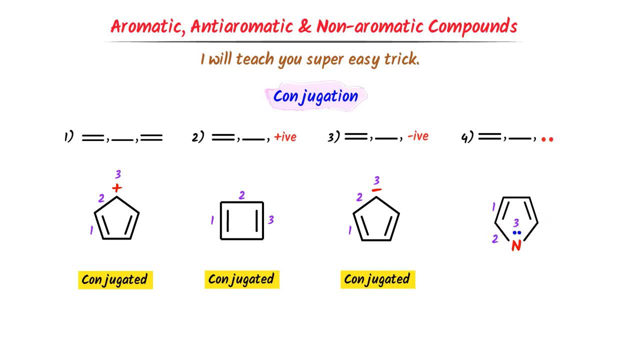 I write 1,, 2,, 3.. This organic compound follows the fourth rule, so it is a conjugated organic compound. So note it down, this important example. Now consider these organic compounds. So note it down, this important example. Now consider these organic compounds In this organic 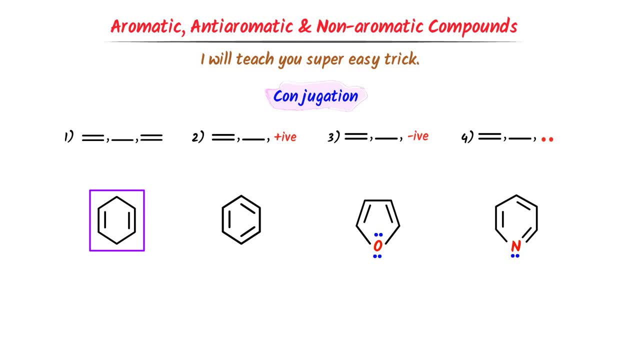 compound, we can see that there is a double bond, single bond, and there is another single bond. I write 1,, 2, 3.. Here, at the third position, there is no negative charge, no positive charge and no lone pair of electrons. It doesn't follow any rule, so it is not a. 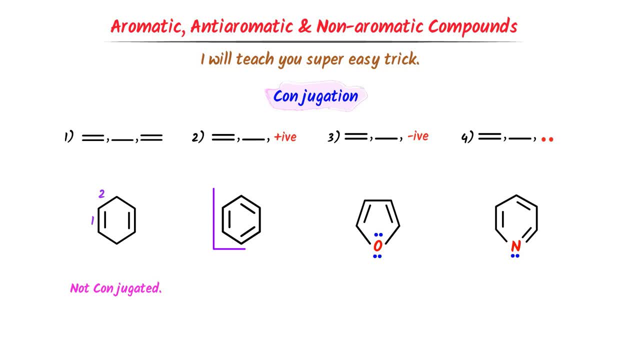 conjugated organic compound. So note it down, this important example. Now consider this organic compound. In this organic compound, we can see that there is a double bond- single. In case of this organic compound, we can see that there is double bond, single bond. and 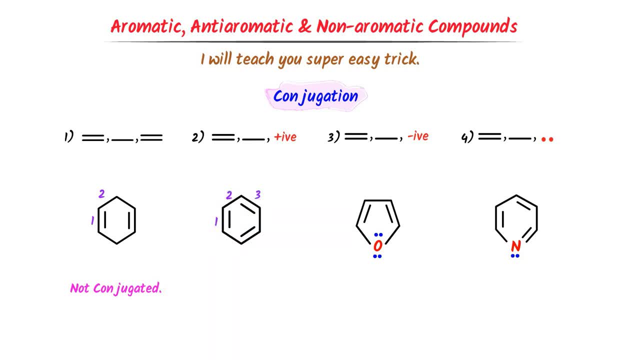 double bond. I write 1,, 2,, 3.. This organic compounds follow the first rule, so it is conjugated organic compound. In this organic compound there are two lone periphelic trones. Remember that this lone periphelic trone is out of the ring. 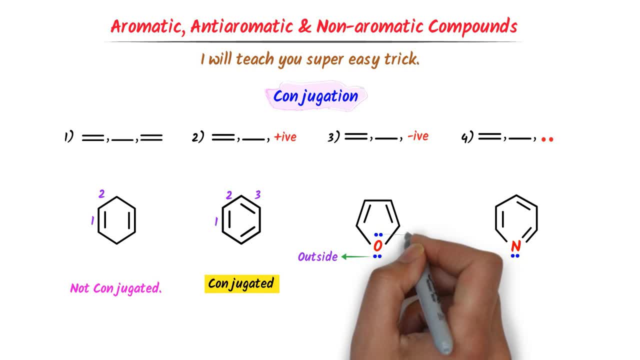 So we say that this lone pear is outside and this lone pear is inside the ring. Remember that if the lone periphelic thon is outside the ring, we do not consider it and the conjugation. Let me repeat it: If the lone periphelic trone is outside the ring, we do not consider it and the conjugation. 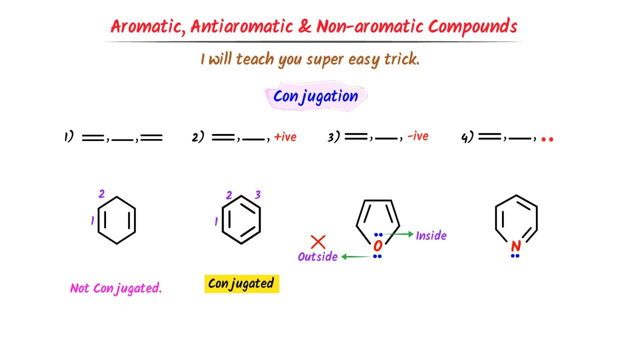 We only consider the lone periphelic trone which is inside the ring, So this stations you take the long approximately take only 1 tone from the whole 몸 2 by the power departure of each of the 3 atoms. 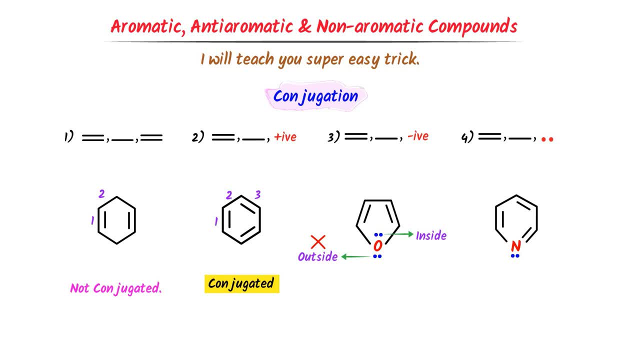 Noety organic compound contains double bond, single bond and a lone pair of electrons. I write 1,, 2, 3.. This organic compound follows the fourth rule, So it is conjugated organic compound. Lastly, in this organic compound this lone pair of electron is outside. So this lone pair of 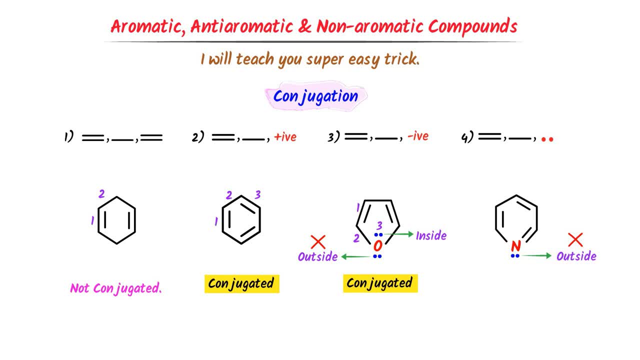 electron doesn't participate in the conjugation, So we do not consider it because it is outside the ring. We can see that this organic compound contains double bond, single bond and double bond. I write 1,, 2,, 3.. This organic compound follows the first rule, So it is conjugated. 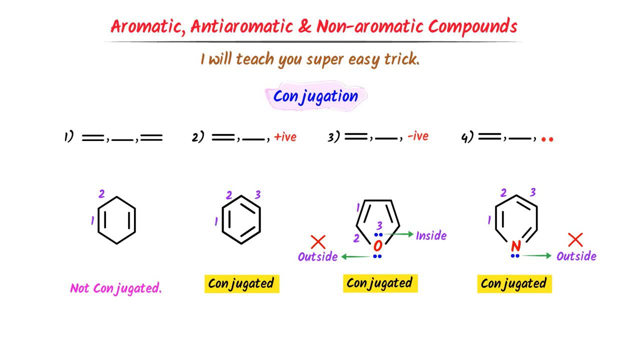 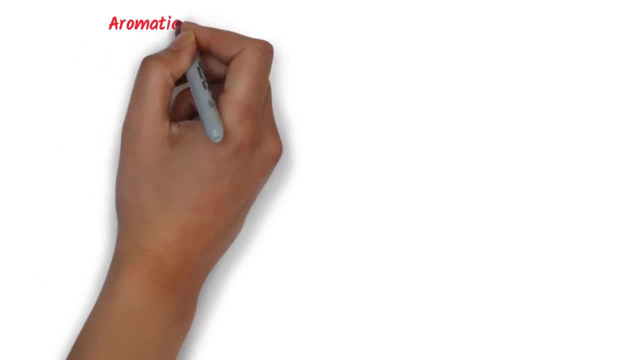 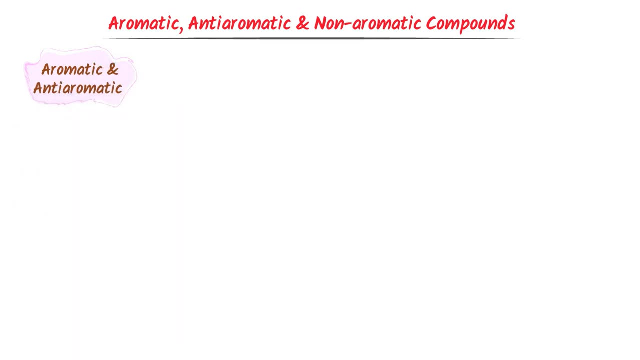 organic compound. Just note it down, this easy method to find the conjugation of any organic compound. Now let me teach you the basic concept of aromatic, anti-aromatic and non-aromatic compound. Aromatic compounds and anti-aromatic compounds are those compounds which are cyclic conjugated. 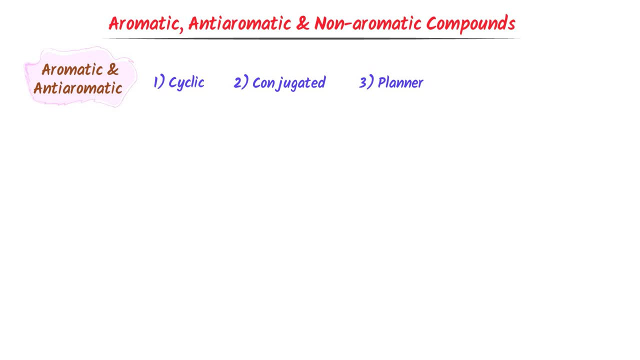 and having planar shape. By planar shape I mean they must have 2D shape or they must have sp2 carbon. Remember that those carbons are sp2 hybridized if they contain only double bond. On the other hand, non-aromatic compounds. 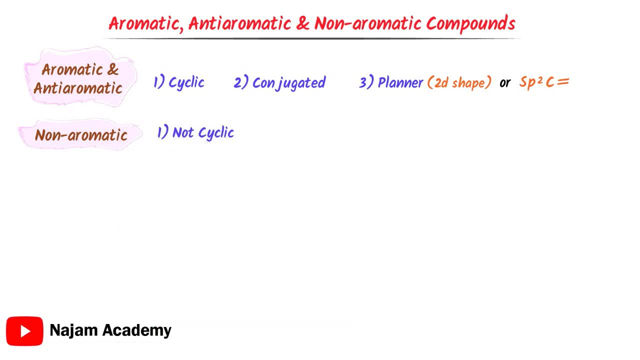 are those compounds which are not cyclic, are not conjugated, For example. consider these organic compounds. We can see that this organic compound is cyclic, So the first condition is fulfilled. Secondly, we can see that it contains double bond, single bond. 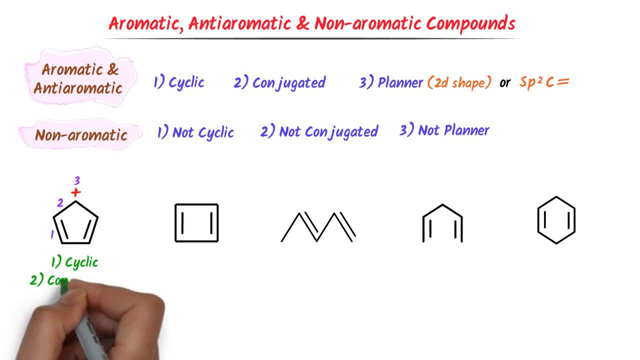 and positive charge. So this organic compound is also conjugated with the therapy solution. So let's now look at the Avenue confusion. Finally, since we described earlier the evolutionary, this is a planar organic compound. So all the three conditions are fulfilled. So this organic 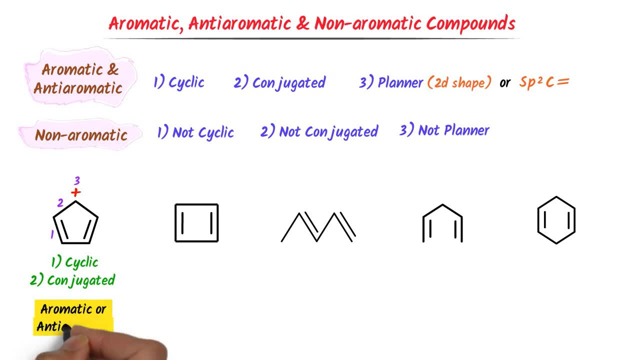 compound is either aromatic compound or anti-aromatic compound. Secondly, this organic compound is cyclic. It contains double bond, single bond, double bond, So it is also conjugated. Thirdly, it is a planar organic compound because it contains a carbon having sp2 hybridization. 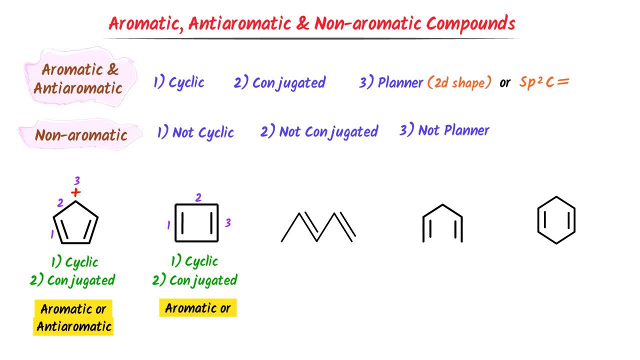 So this organic compound is either aromatic organic compound or anti-aromatic compound. Thirdly, we can see that this is not cyclic organic compound, So it is non-aromatic compound. Fourthly, this organic compound is not cyclic, So it is also non-aromatic compound. Fifthly, we can see that this is a cyclic organic 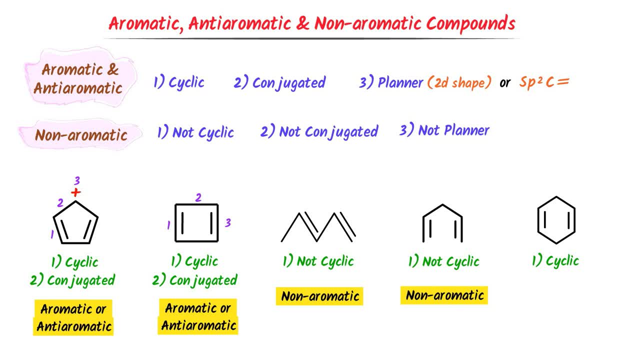 compound. So the first condition is satisfied. Now we can see that it contains double bond, single bond. At the third position, there is no lone pair of electron, no negative charge and no positive charge. So this organic compound is not conjugated. Therefore this: 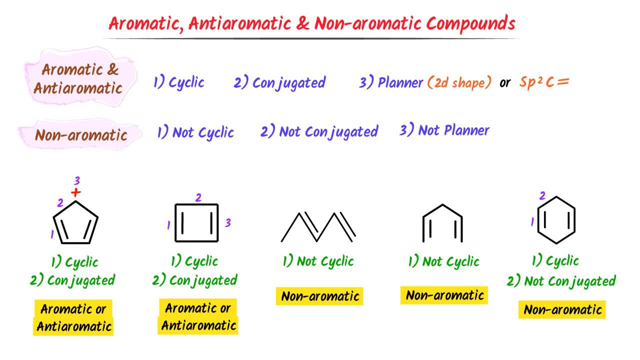 is non-aromatic compound. Just remember that if a compound is cyclic, conjugated or planar, it is either aromatic compound or anti-aromatic compound. If a compound is not cyclic, not conjugated or not planar, it is non-aromatic compound. 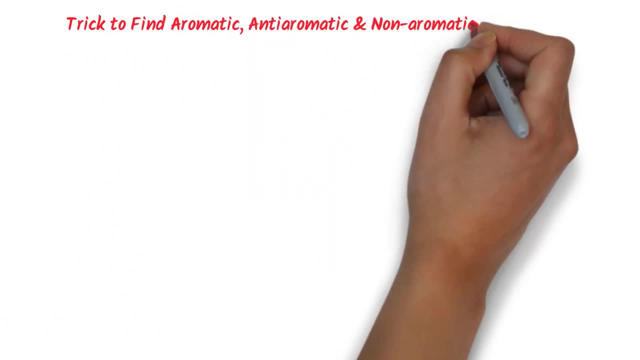 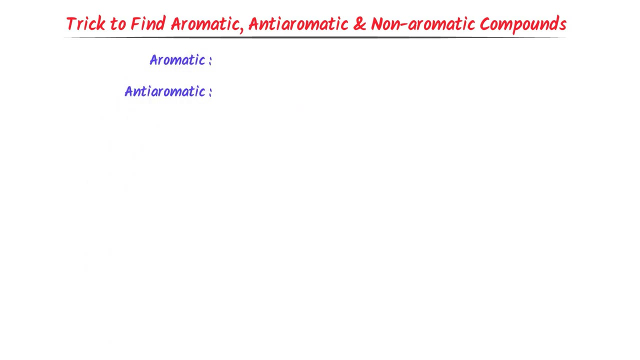 Now I will teach you the super easy trick to find aromatic compounds and anti-aromatic compounds. For aromatic and anti-aromatic compounds I write 2, 4.. Now- listen carefully- I add 4 to these two successively: 2 plus 4 is equal to 6,. 6 plus 4 is equal to 10,. 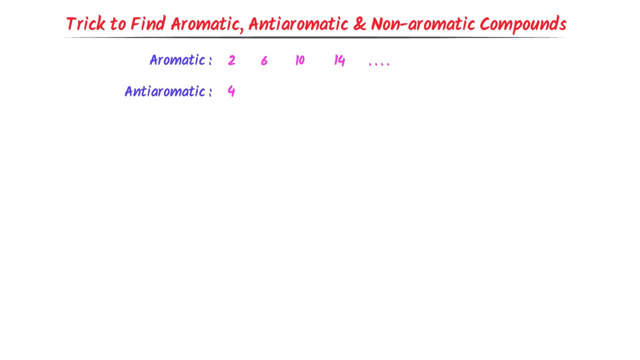 10 plus 4 is equal to 14.. Similarly, I add 4 to these four. successively: 4 plus 4 is equal to 8,. 8 plus 4 is equal to 12.. 12 plus 4 is equal to 16.. 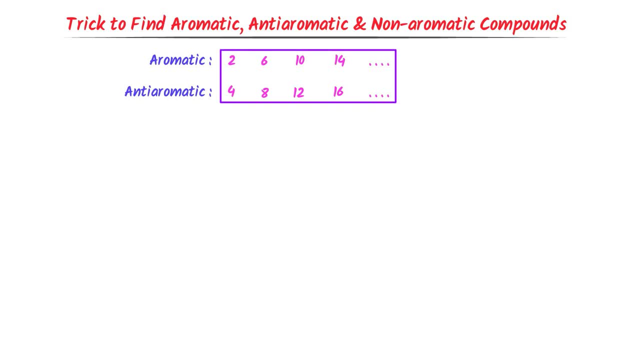 Remember that these 2,, 6,, 10,, 14,, 4,, 8,, 12,, 16 represents the number of pi electrons. We already know that aromatic compounds are those compounds which has 4n plus 2 pi electrons. 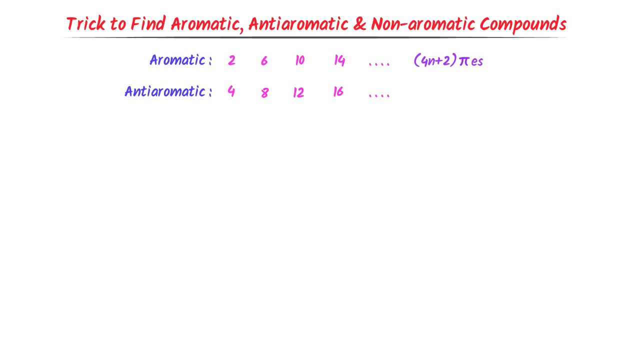 while anti-aromatic compounds are those compounds which have 4n pi electrons. Also note it down. Remember that for each double bond, I will write 2 electrons. For each negative charge, I will write 2 electrons. For each long pair of electrons, I will write 2 electrons. 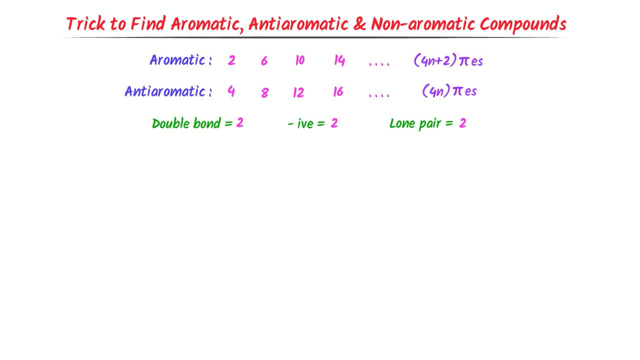 Remember that for positive charge I do not write any electron. Now consider these organic compounds. We can see that this organic compound is cyclic. Secondly, this organic compound contains double bond- single bond and double bond, So it is also conjugated organic compounds. 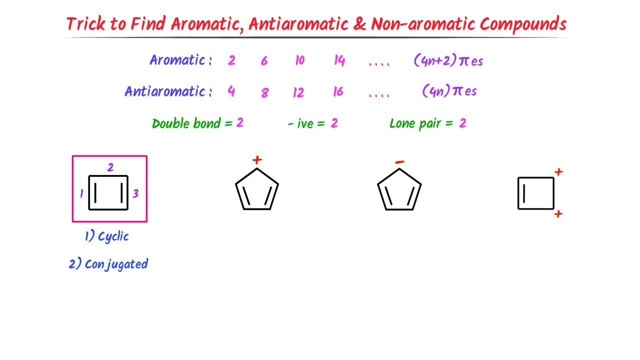 Now inside the ring there are 2 double bonds. We already know that for each double bond I have to write 2 electrons. So I write 2 electrons plus 2 electrons, which is equal to 4 electrons. We know that. 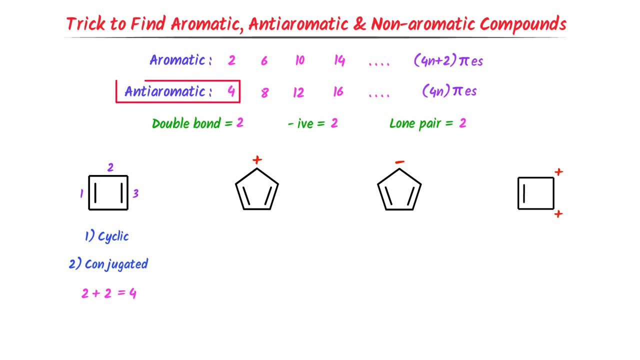 We know that If organic compound contains 4 electrons, it is anti-aromatic. So this organic compound is anti-aromatic. Secondly, we can see that this is cyclic organic compound. Now here there is double bond, single bond and positive charge. 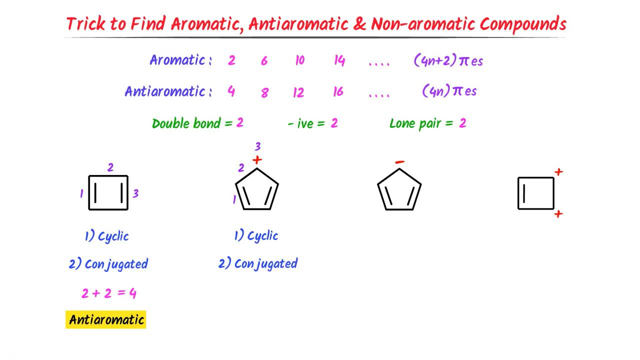 So this organic compound is conjugated Inside the ring there are 2 double bonds. I write: 2 plus 2 is equal to 4 electrons. So this organic compound is anti-aromatic. We know that. We know that If organic compound contains 4 electrons it is anti-aromatic. 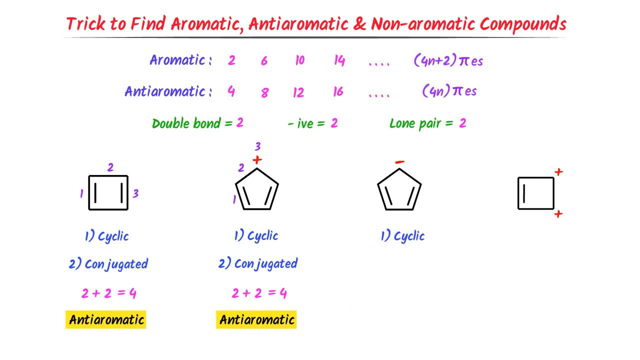 Thirdly, this is cyclic organic compound. Here this organic compound contains double bond, single bond and negative charge, So it is conjugated organic compound. We can see that this ring contains two double bonds, So I write 2 plus 2.. 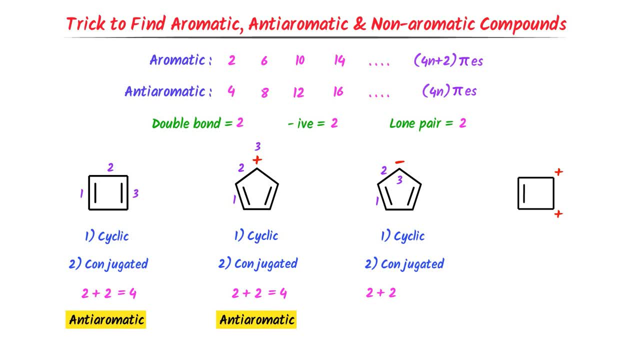 But why? But wait a minute. this cyclic organic compound also contain negative charge. We already know that if a ring contains negative charge, for each negative charge we have to put 2 electrons. So I write here 2 electrons. now, 2 plus 2 plus 2 is equal to 6 electrons. 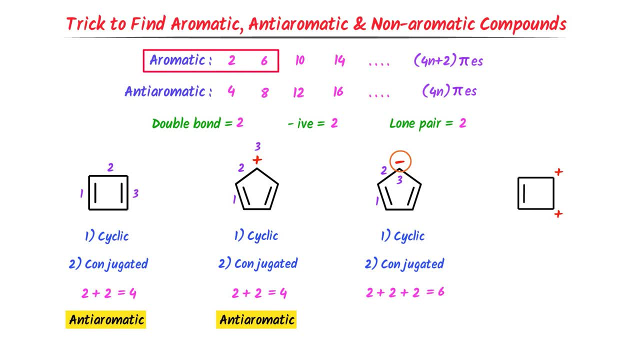 We know that if a compound contains 6 electrons, it is aromatic. So this compound is aromatic. Fourthly, this is cyclic organic compound. Also, it contains double bond, single bond and positive charge, So it is conjugated. We know that for each double bond we have to write 2 electrons. 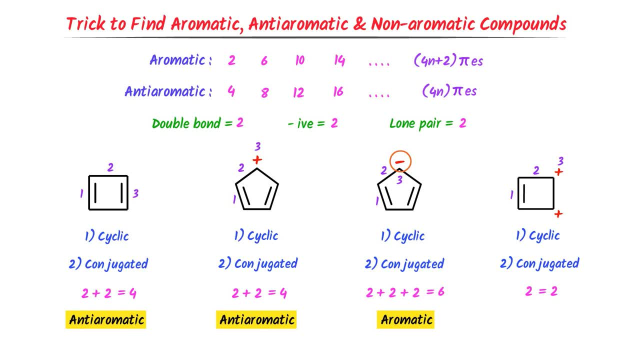 Now, 2 electrons is equal to 2 electrons. We know that if a compound contains 2 electrons, it is aromatic, So this compound is aromatic. Hence noted down these basic examples of aromatic compounds and anti-aromatic compounds. Now consider these aromatic compounds. 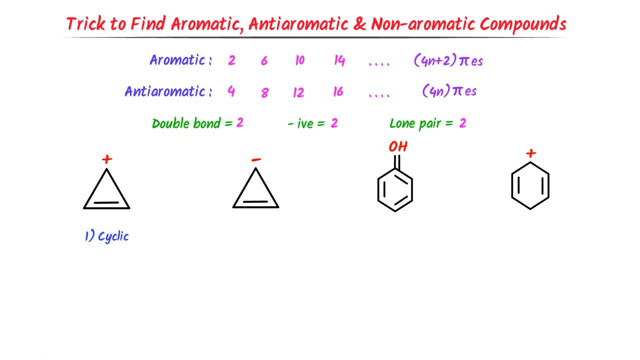 This aromatic compound is cyclic. Secondly, it is also conjugated. It contains one double bond, So I write here 2 electrons. According to the rule, if a compound contains 2 electrons, it is aromatic. So this compound is aromatic. 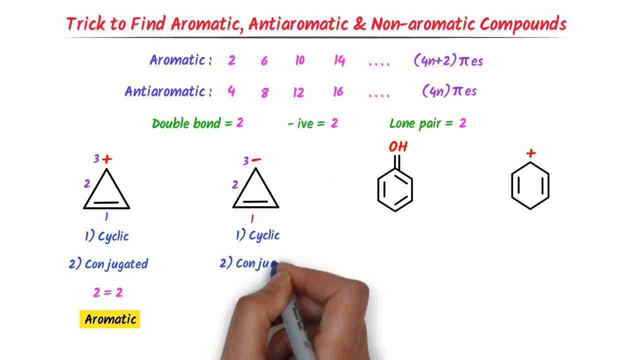 Secondly, it is cyclic and it is conjugated. For this double bond, I write 2 electrons. For this negative charge, I write 2 electrons. 2 plus 2 is equal to 4 electrons. According to the rule, if a compound contains 4 electrons, it is anti-aromatic. 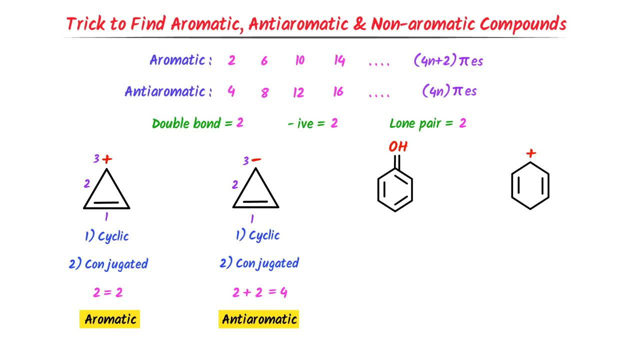 So this organic compound is anti-aromatic. So this organic compound is anti-aromatic. Thirdly, this organic compound is cyclic and it is also conjugated. We can see that this organic compound contains 3 double bonds. I write: 2 plus 2 plus 2 is equal to 6 electrons. 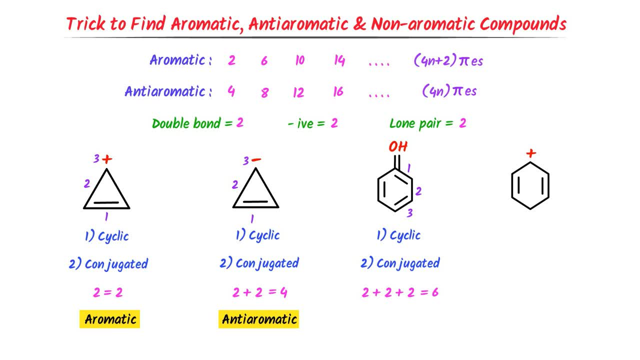 According to the rule 6 electrons means aromatic, So this organic compound is aromatic. Fourthly, this organic compound is cyclic And this organic compound is also aromatic, So this organic compound is cyclic. 4 electrons constitute about 5 electrons. 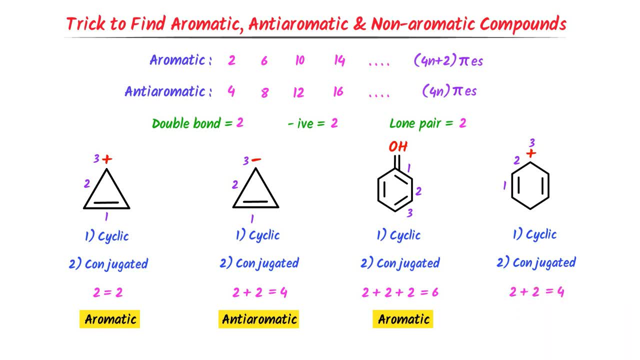 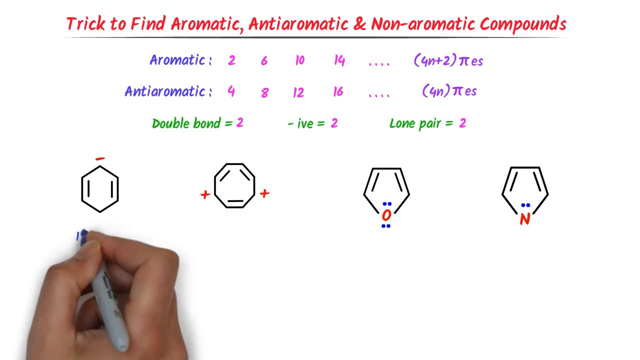 So 4 electrons constitute about 2. Now consider these organic compounds. We can see that this organic compound is cyclic. It is also conjugate organic compound. Let me ambient andetas organic compound. This organic compound: 2 double bonds. We can write 2 plus 2 equal to 4 electrons. 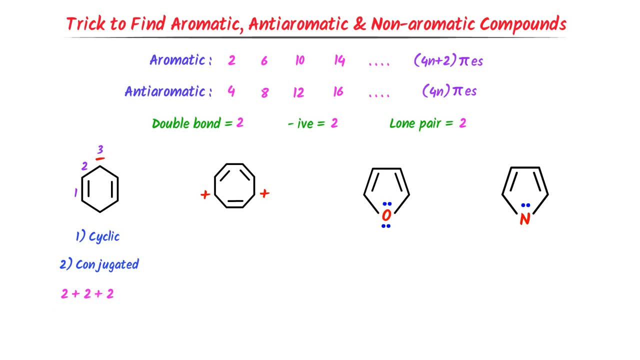 bonds, I write 2 plus 2.. For this negative charge I write 2 electrons. Now 2 plus 2 plus 2 is equal to 6 electrons. We know that 6 electron means aromatic compounds, So this is aromatic compound. 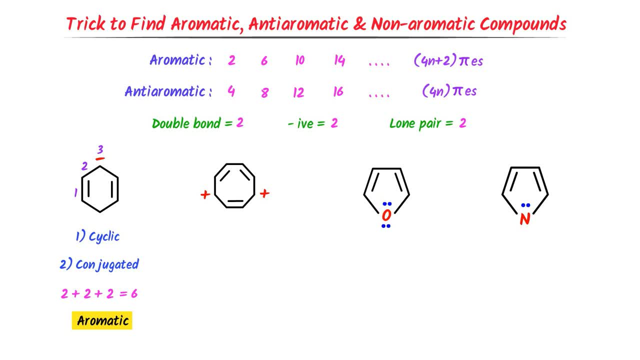 In case of this organic compound, we can see that this is cyclic organic compound and it is also conjugated organic compound. There are three double bonds. I write 2 plus 2 plus 2 is equal to 6 electrons, So this organic compound is aromatic compound. In case of this organic 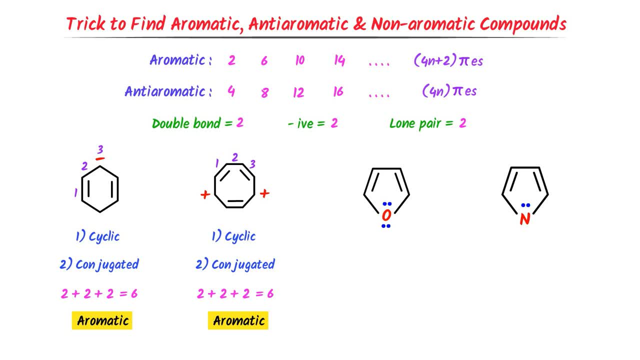 compound. remember that this organic compound is known as furon. It is cyclic and it is conjugated. We can see that this organic compound contains two lone parafflectrons. This lone parafflectron is outside the ring, So we do not consider it. This lone parafflectron is inside the ring. 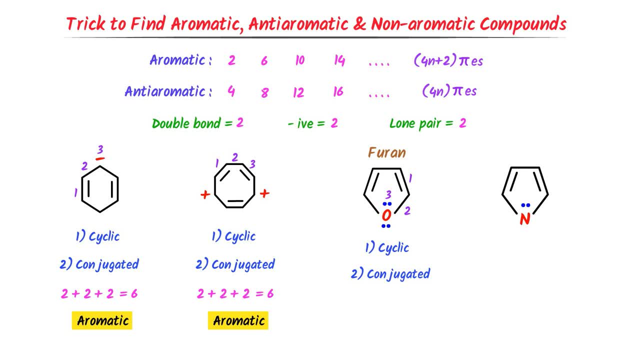 So we consider this lone parafflectron, So it is also conjugated organic compound. Now there are two double bonds. I write 2 plus 2.. For this lone parafflectrons I have to write 2.. Now 2 plus 2 plus 2 is equal to 6 electrons. So furon is an aromatic organic. 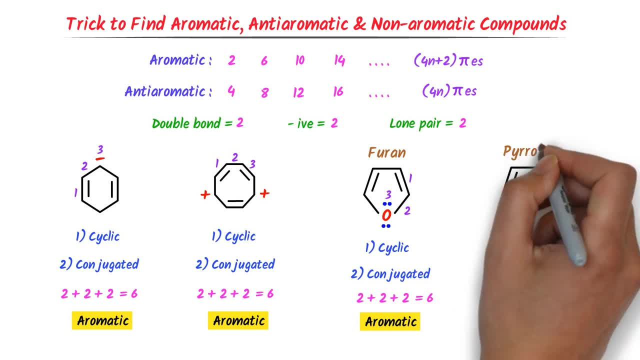 compound. This organic compound is known as pyrrole. It is cyclic organic compound and it is conjugated organic compound. There are two double bonds: I write 2 plus 2.. For this lone parafflectrons, I write 2, which is equal to 6 electrons. So pyrrole is aromatic organic compound. 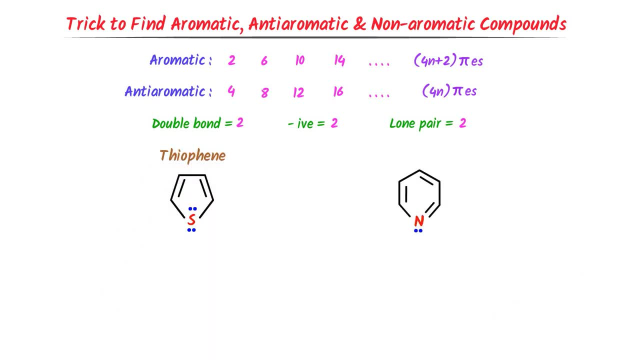 This organic compound is known as thiophene. It is cyclic organic compound And it is also conjugated organic compound. Remember that this lone parafflectron is outside the ring, So we do not consider it in the conjugation. There are two double bonds. I write. 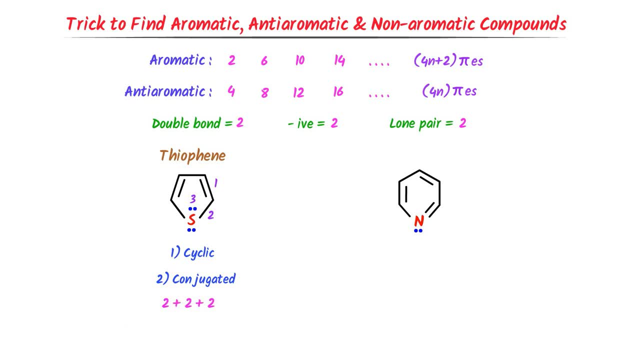 2 plus 2.. For this lone parafflectron I write 2, which is equal to 6 electrons. We know that if there are 6 electrons it is aromatic compound. Lastly, pyrrole is aromatic organic compound. 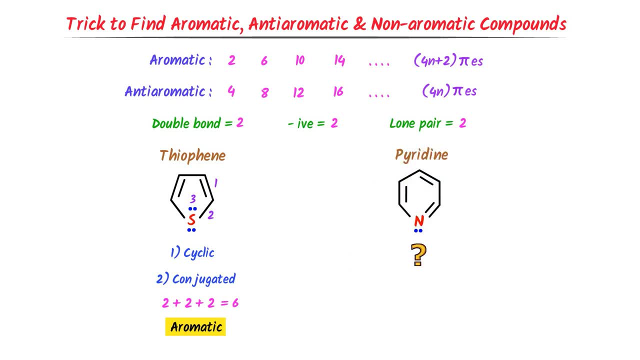 Lastly, consider pyridine. Pause the video and try to find it. Either it is aromatic compound or anti-aromatic compound. Well, it is cyclic organic compound. Secondly, this lone parafflectron is outside the ring, So we do not consider it. We can see that it is a conjugated organic compound. 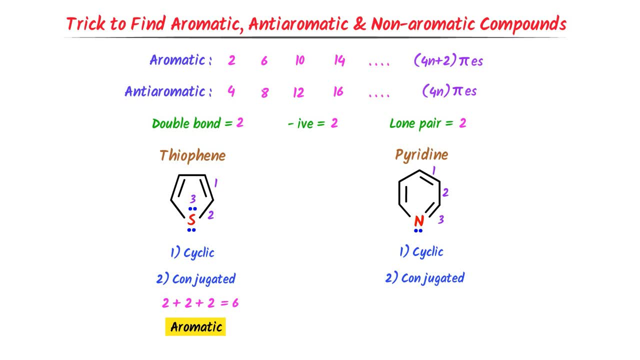 There are three double bonds. For these three double bonds I write 2 plus 2 plus 2 plus 2, which is equal to 6.. Here remember that for this lone parafflectron I do not write 2 electrons because it is not participating in conjugation. 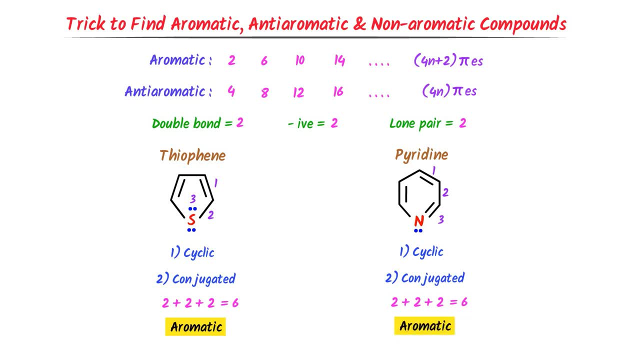 6 electron means aromatic compound, So this is aromatic compound. Let's note down all these important examples of aromatic compounds and anti-aromatic compounds. Now let me tell you about pyrrole. Pyrrole is aromatic organic compound, So pyrrole is aromatic. 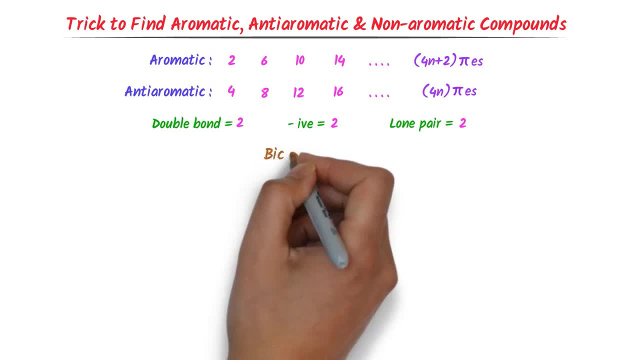 compound and it has two pyrrole-cons, 유튜�ve ribose properties. In this one mangosteen problem, pyrrole means that the pyrrole is aromatic organic compound, So for each one mangosteenан anthelium or pyrrole gives the pyrrole of pyrrole or 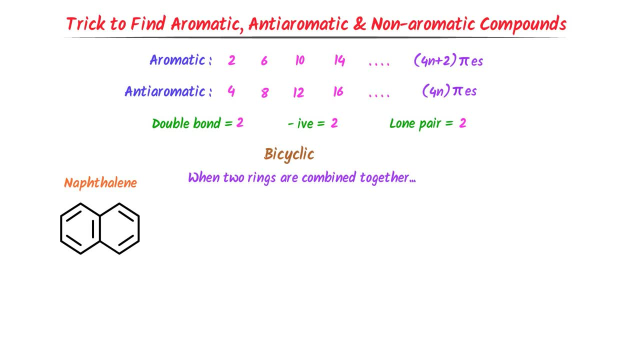 pyrrole. the ability to Ó Cecil 2 Tri implies This one means that at this point of game we can užire it, So we can write it as pyrrole. Orbene, that it is a string, Hey. 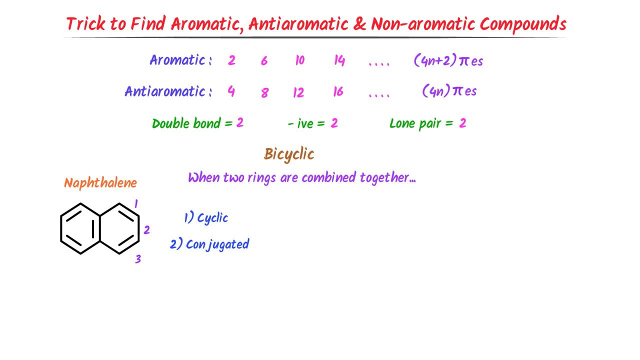 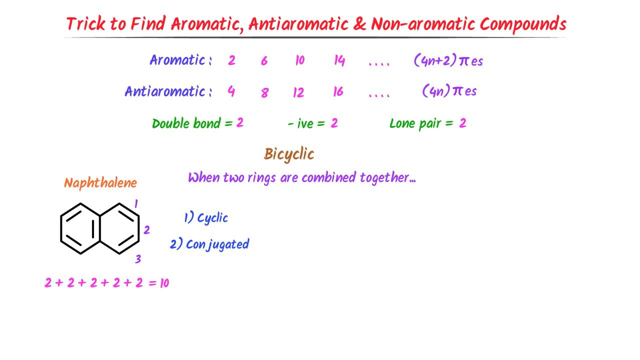 According to the rule, if a compound contains 10 electrons it is aromatic compound. So naphthalene is aromatic compound. Secondly, consider pentylene. It is a bicyclic organic compound because two rings are fused together or joined together. 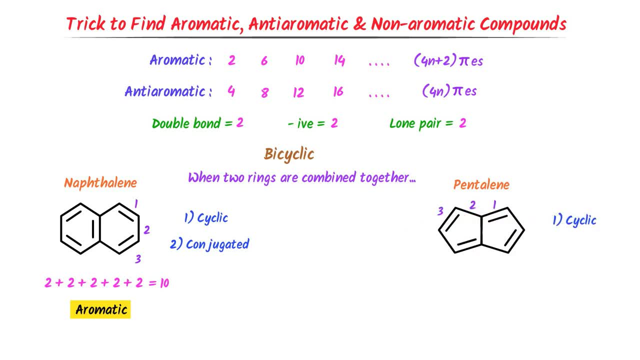 This is cyclic organic compound and it is a conjugated organic compound because it contains alternate single and double bonds. Now, inside these two rings, there are four double bonds. I write 2 plus 2 plus 2 plus 2, which is equal to 8 electrons. 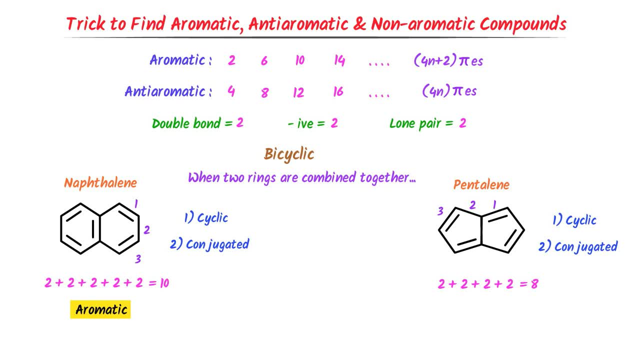 According to the rule, if a compound contains 8 electrons, it is anti-aromatic compound. So this organic compound is anti-aromatic compounds. Thus, note it down, these two important bicyclic organic compounds. Now we will learn the aromatic and anti-aromatic compounds and biphenyl organic compounds. 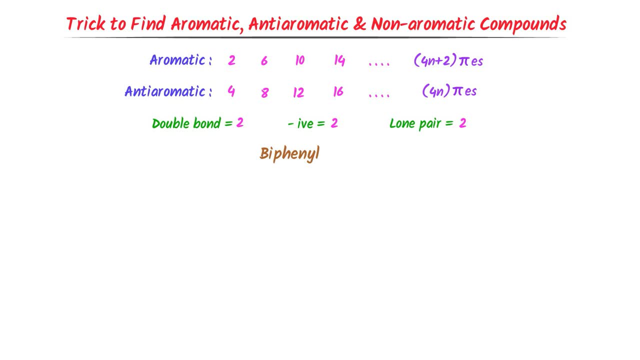 Remember that biphenyl organic compounds are those compounds. when two phenyl groups are in the same group, They are bonded together, For example. consider this: biphenyl organic compounds. In case of biphenyl, we will individually check each ring. 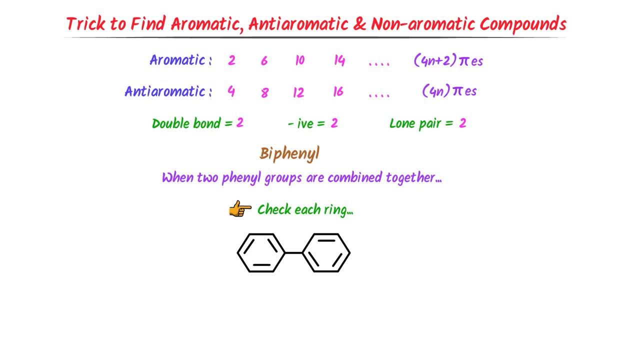 Either it is aromatic or anti-aromatic. In case of this ring, it is cyclic and it is conjugated. It contains three double bonds. I write 2 plus 2 plus 2, which is equal to 6 electrons. So this ring is aromatic and anti-aromatic. 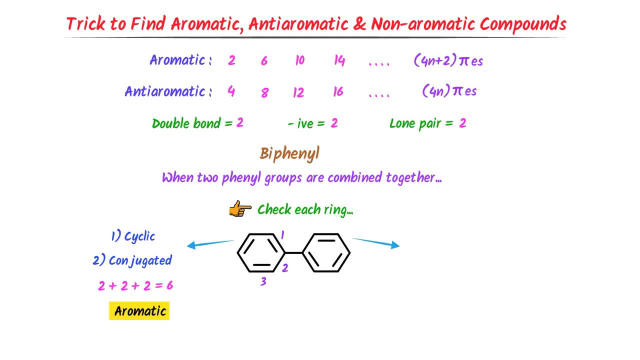 is aromatic ring. In case of this ring, it is also cyclic and it is conjugated. It contains three double bonds. I write 2 plus 2 plus 2 is equal to 6 electrons, So this ring is also aromatic. Thus both the rings are aromatic. We call this biphenyl organic compounds, as 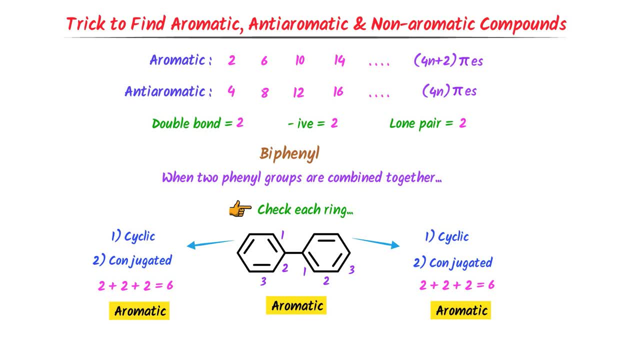 aromatic organic compound. Remember that overall it contains six double bonds. Six double bonds means 12 electrons. Then we can say that it is anti-aromatic, But this is wrong Because we have to individually check each ring. either it is aromatic or anti-aromatic. So remember this.